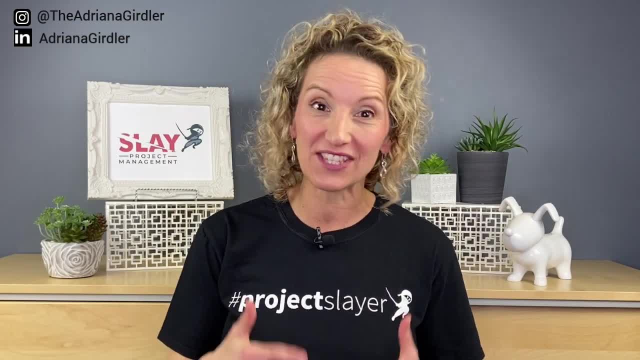 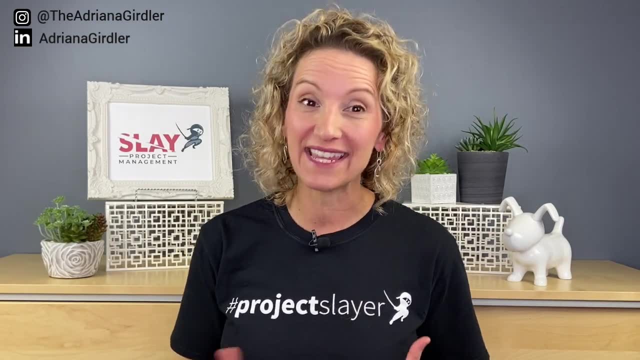 always look at it, juggle it around and know that it is an art. Through practice you're going to get really good at it. So on my last point, be kind to yourself. This is an art. It's not something that comes naturally to some people. Sometimes you have to. 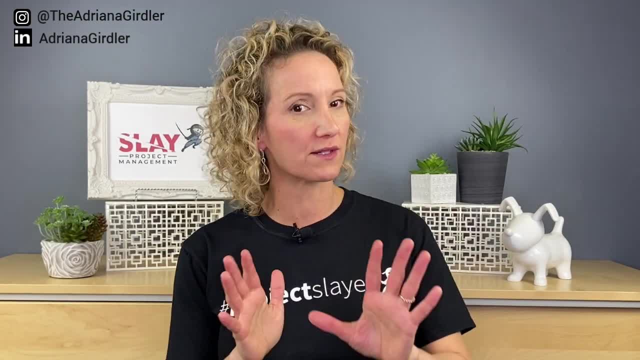 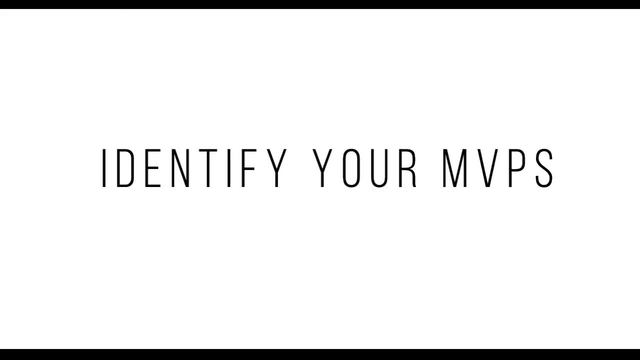 work with it and you just have to practice, But I promise you learn this: prioritize properly and it's really going to make a big difference. Identify your MVPs- This is your most valuable players on each of your projects. Identify your MVPs: This is your most valuable players on each of. 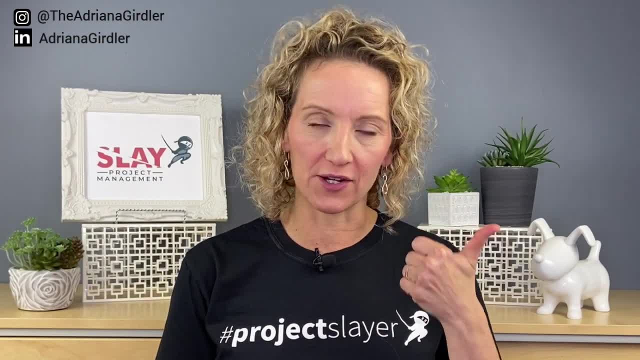 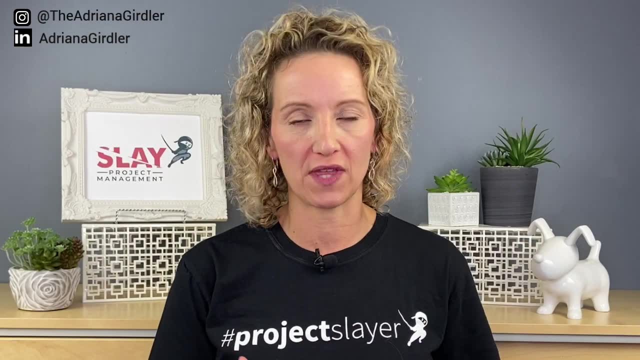 your teams. This becomes critical, just like I said, with the art of prioritization. Your team members are going to be executing stuff, So you need to know who you can go to. You want to make sure that there's going to be certain key people that are probably higher in rank from a standpoint. 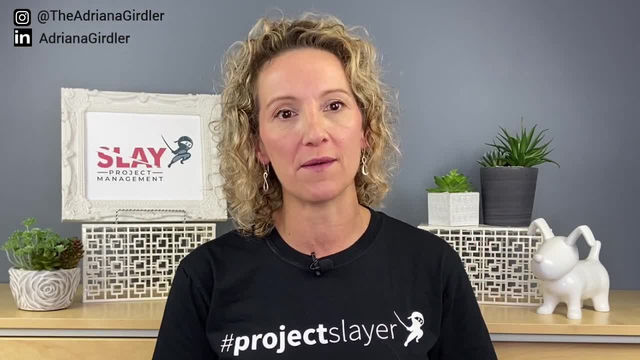 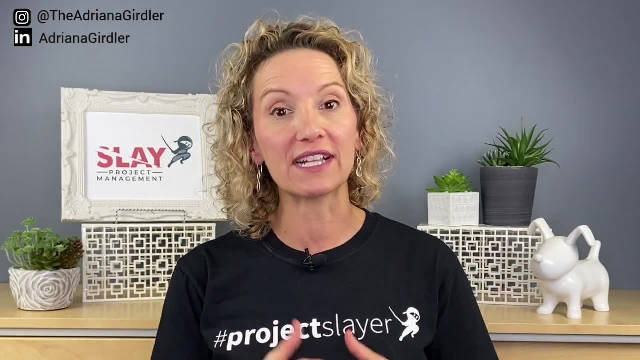 of the activities they have to do. So really connect with them so that you can have an understanding as to what they're doing. Maybe have a little bit more one-on-one relationships so that you can be very clear with the reporting structure you want from them. It just makes your 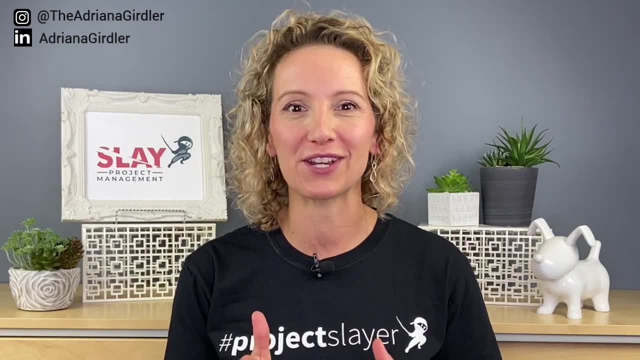 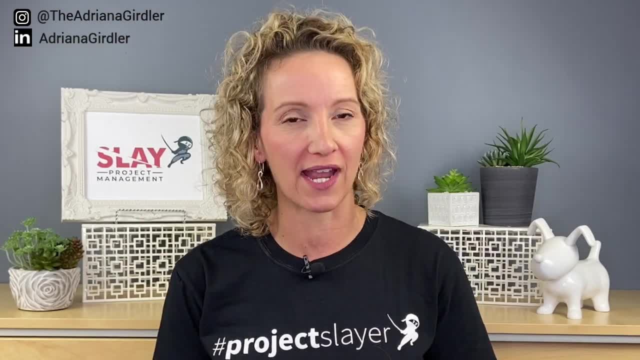 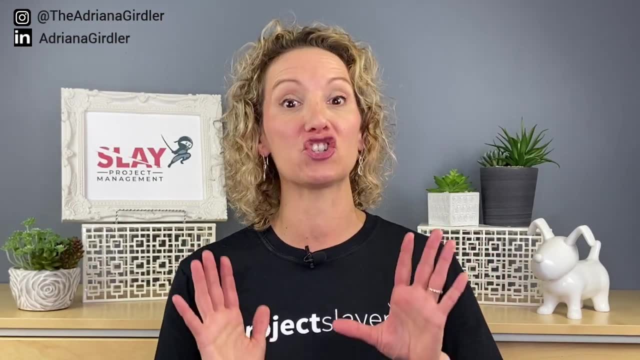 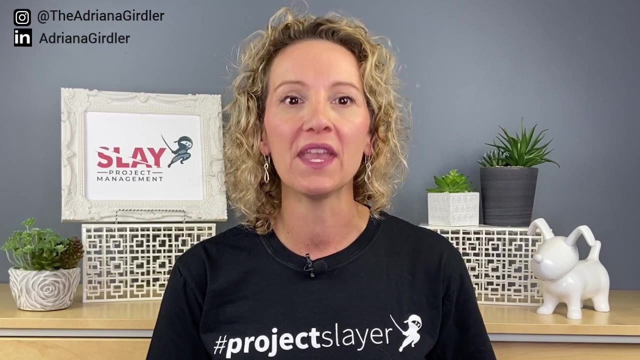 communication to ensure that things are on track Because, again, you're juggling, You have multiple projects going on, So the key to that is delegating and ensuring that they are doing what they're doing. Don't micromanage. Delegate and set things up with a structure And that really helps. 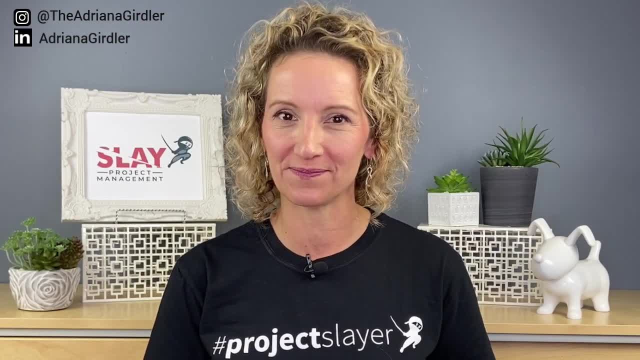 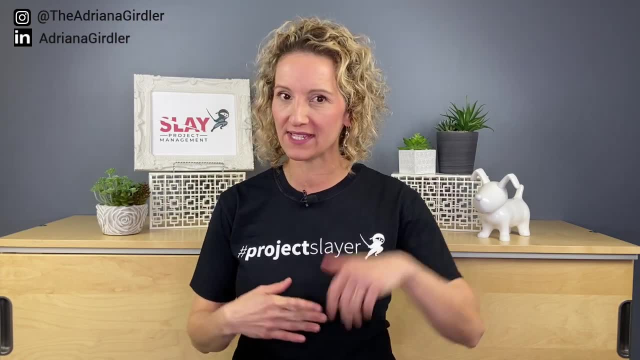 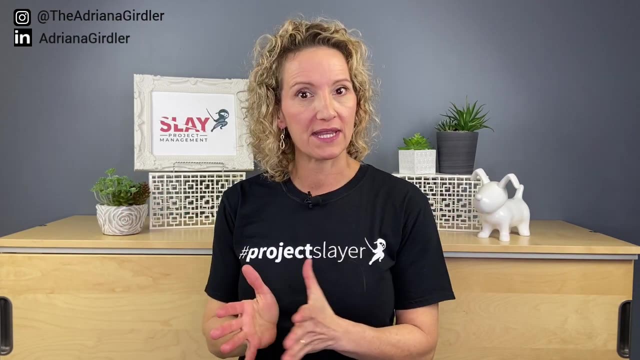 tremendously to managing multiple projects. Paperwork is your BS. Okay, You're probably gathering, now that there's a theme going on here, that what we said with prioritization, MVP and now we're talking about documentation, Absolutely Your project plan becomes critical, and even more so when you're doing multiple projects. 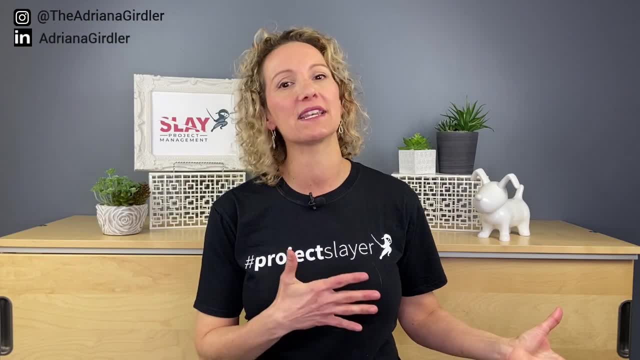 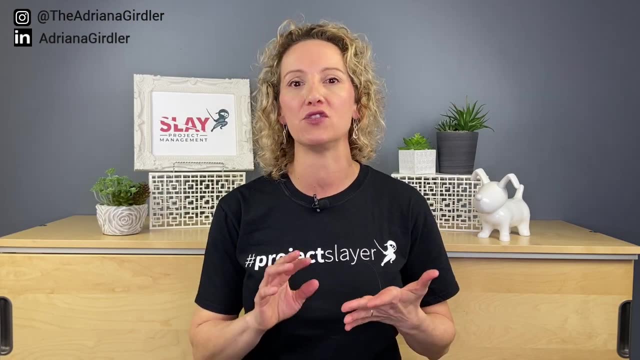 So if you've done your due diligence, you've done your planning upfront, then it's going to make your life a lot easier because you've established expectations, you've established ways of working and you formalize those updates And you're managing of. 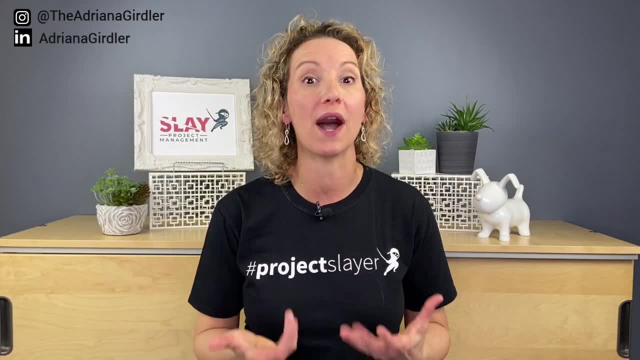 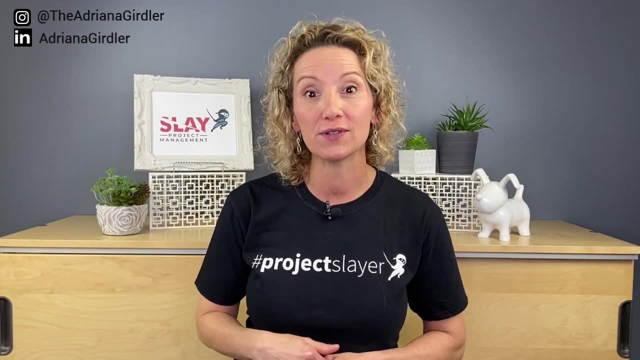 documentation is just where you can go to to confirm things, remind people as the projects are progressing, And it's also a place for your MVPs to go to. And what's really cool, too, is part of that major timeline that you're creating for all your projects is again. 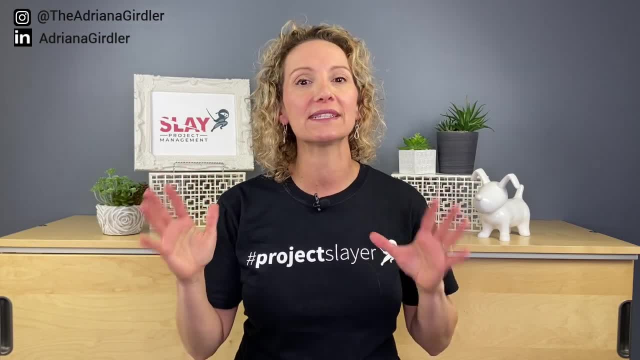 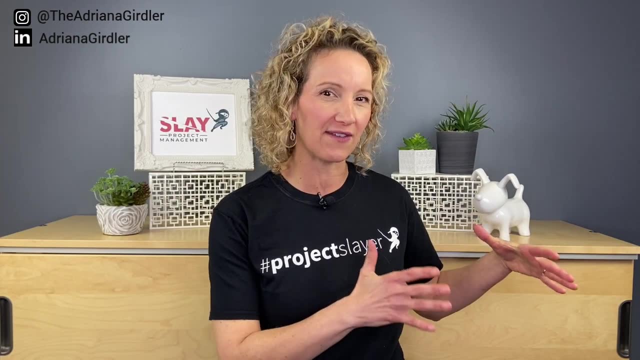 going to be documented. You're not keeping that in your head. it just makes life a lot easier. So do that work. That's due diligence on your part. Yes, It's a little bit of heavy lifting upfront, but so worthwhile in the life cycle of the project. But the most important thing, 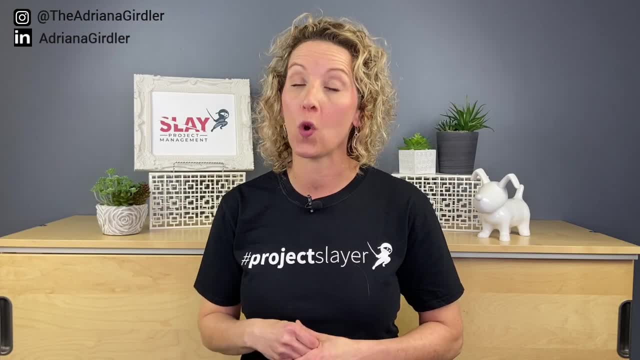 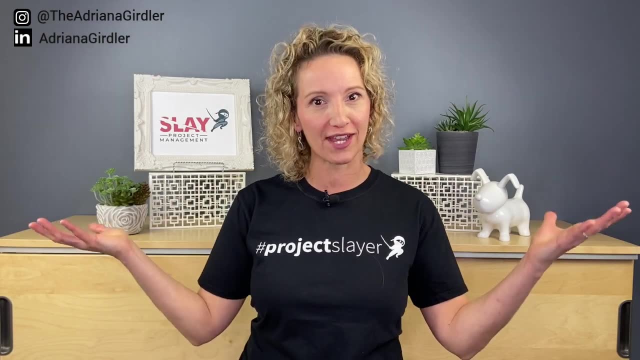 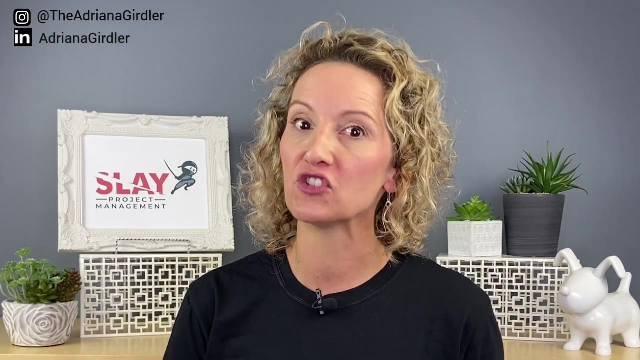 project as you're executing. It's just going to make your life a whole lot easier. So do your paperwork. Do not ignore it, particularly when you're running multiple projects. Duplicate success, All right. One thing I've learned over the years: doing the efficiency: 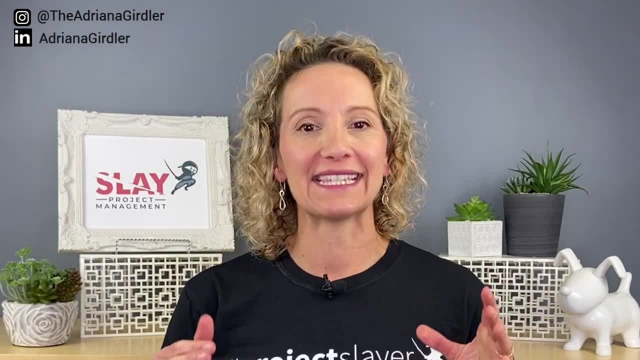 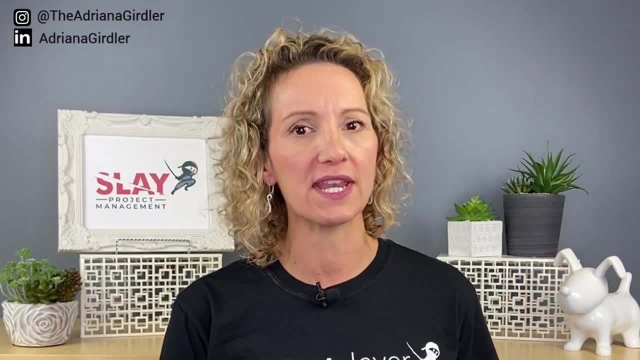 work that I do, the engineering work that I do, is that there's patterns to everything, And that's the beauty of standardization in the efficiency world is you can see the patterns. Now you may have some customization that you do, depending on what it is that you're. 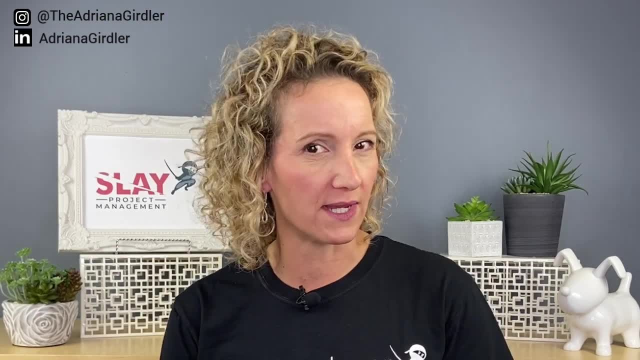 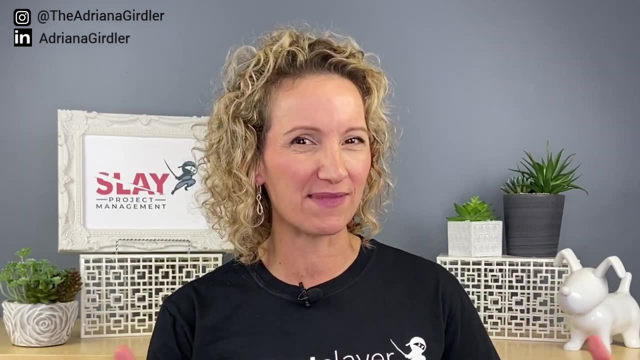 working on, but you don't want to reinvent the wheel, So have those checklists. have standard templates. If every project you're working on has the same set of documentation, it's going to make your life a lot easier in managing those multiple projects You're. 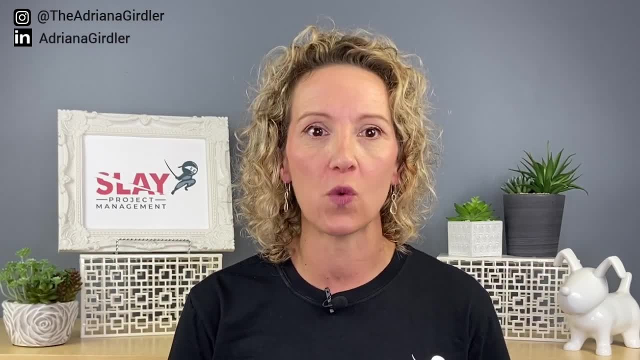 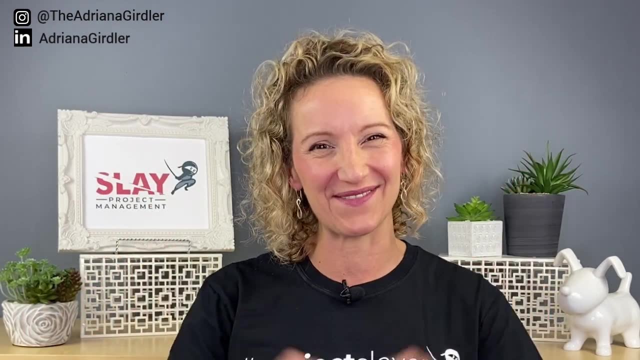 not doing something special or different for each one and then trying to figure out: what did you do for that project or this project? It's the same standard. Yeah, It's the same standard recipe. right? It's the recipe for success. So ensure you duplicate. 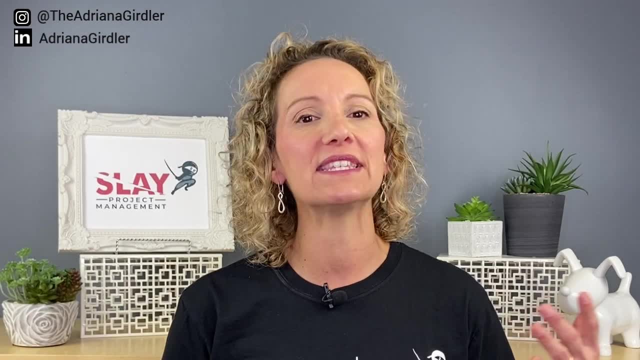 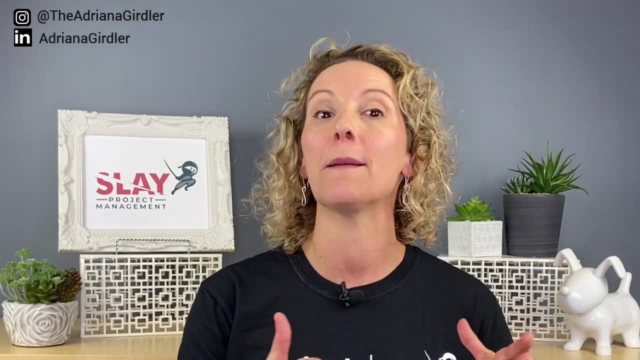 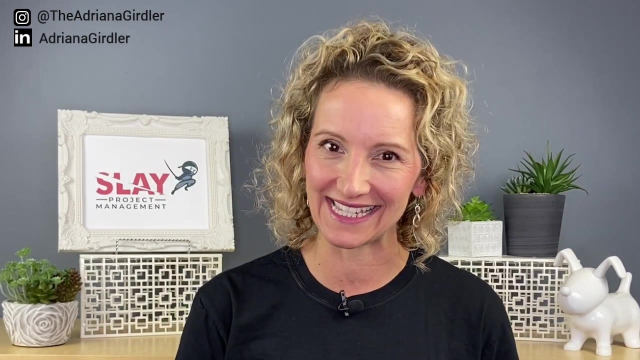 that success. Learn from your past projects. If something didn't work out well, well make sure that you change that moving forward in the future and change all your templates accordingly so you can build off of that with all of your projects. So really learn from each other in regards to the projects. duplicate that success have. 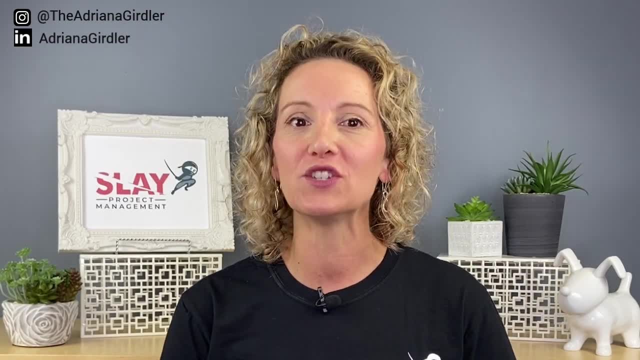 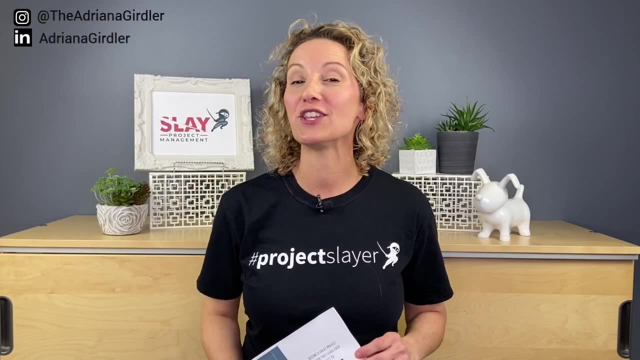 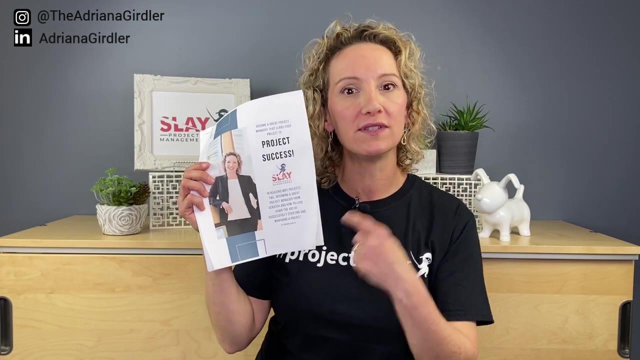 those standard templates and use it for everything. It's going to be a game changer in regards to helping you manage those multiple projects. Okay, Now that you know how to manage multiple projects, I want you to go to the link below and grab this: how to deal with project failures. This is just as important as learning how. 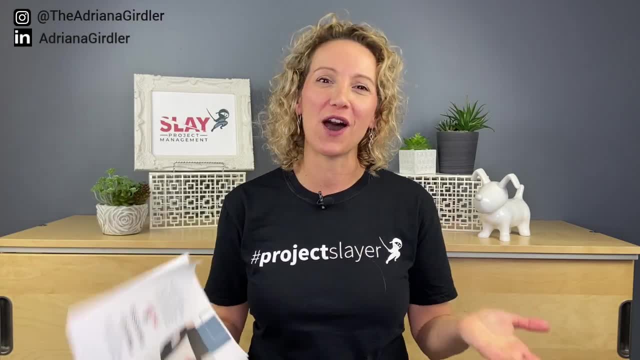 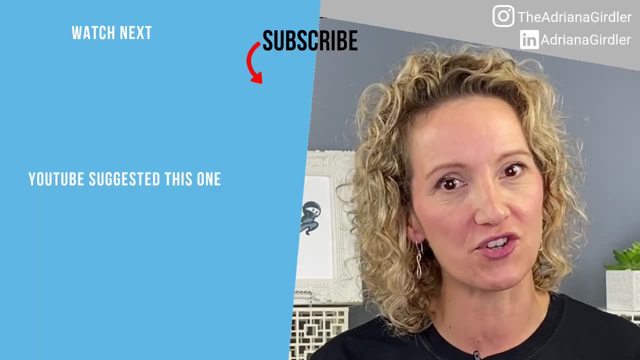 to manage multiple projects, So go to the link below Now. on that note, please like this video, subscribe to my channel and share it with all the friends that you know. If you have any additional tips on managing multiple projects, please put it in the comments below. Until the next time, See ya.